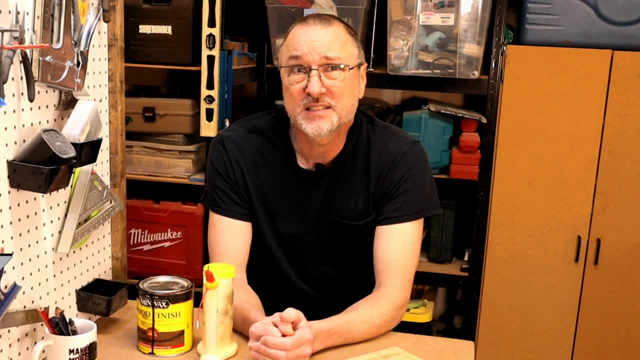 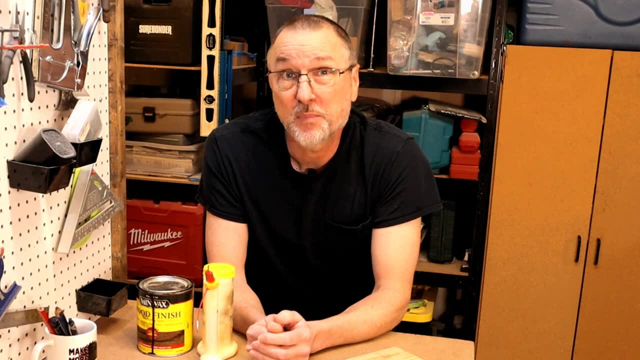 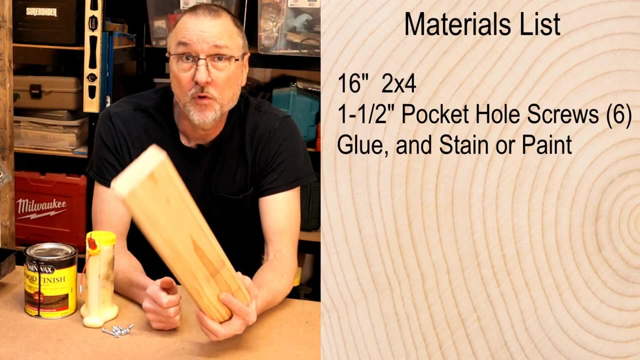 Today's project actually is going to cost about 80 cents to build and it's going to produce a woodworking project worth around 25 bucks- 25 bucks, that's 31 times increase from what you started with and it's not going to take very long: 16 inch 2x4, a few pocket hole screws, some glue. 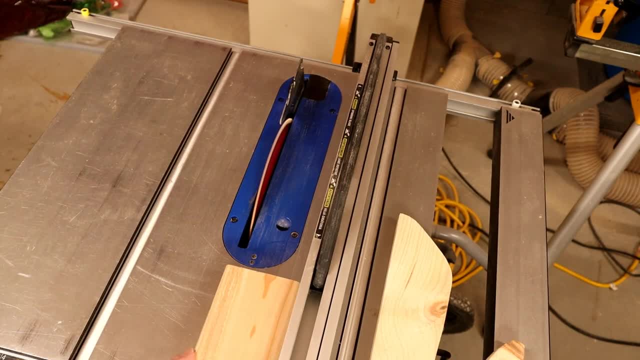 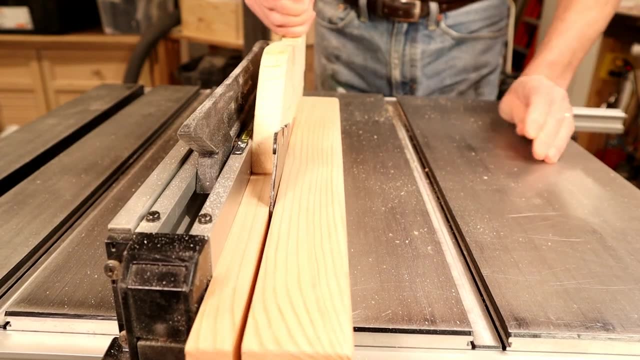 and some stain. Let me show you how it's done. I start here by ripping off the edge of the 2x4, then I set the saw to 3 quarters of an inch and rip four strips. After that I round over all the. 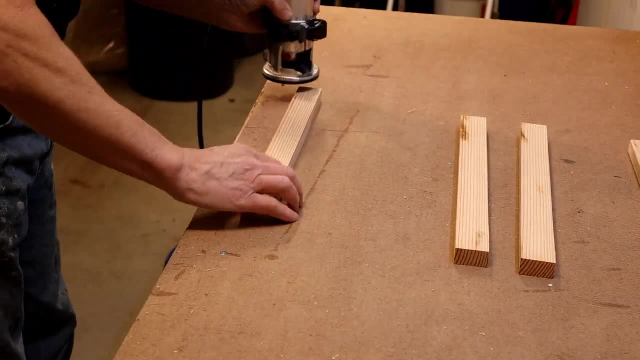 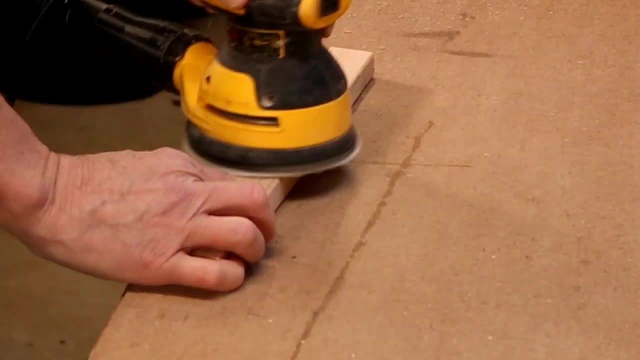 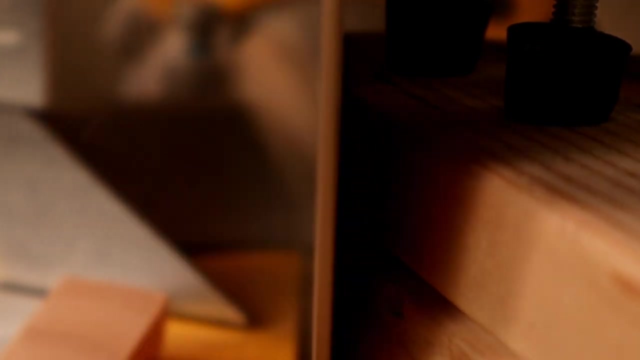 corners of the strips with an 8 inch round over bit on my palm router, Then sand everything down smooth. This is really a very safe and secure way to make these high angle cuts and with a jig being capable of holding both boards in place, you get a precise angle on both boards with just 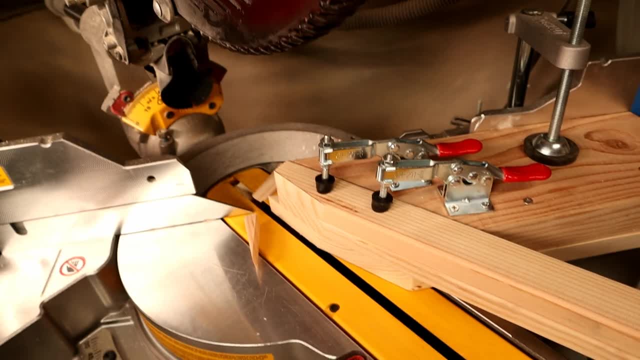 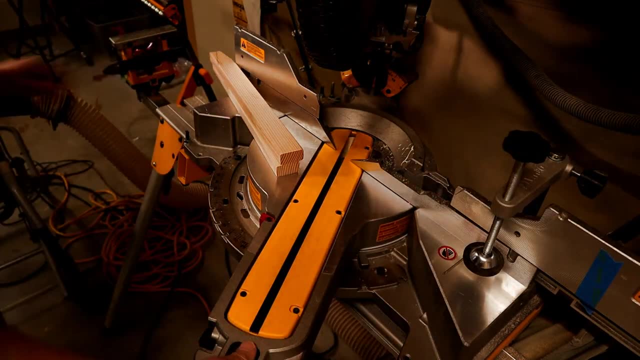 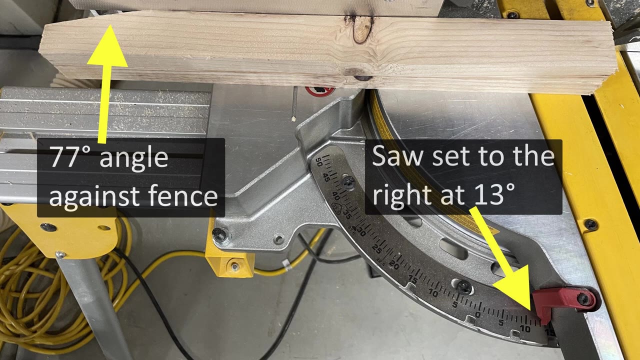 one cut. I had to hold the blade guard up a bit to clear the toggle clamps. However, my hands are nowhere near the blade. Now, once the cut is made, the other ends get placed for a 13 degree cut to the right. The previous 77 degree angle goes against the fence as shown Now. I cut the 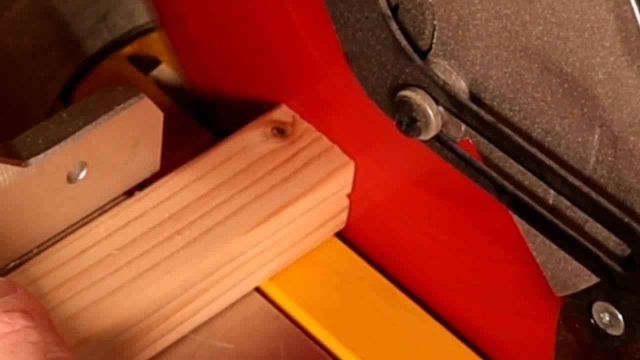 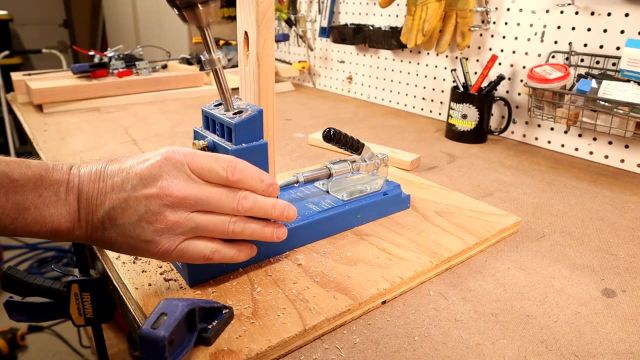 remaining 2 slats in half. I'll use 3 of the four pieces in this project. Each of the three gets a pocket hole at each end, Since they're 3 quarters inch thick. that's what I set the jig to. Now it's just a matter of lining up the rungs with my 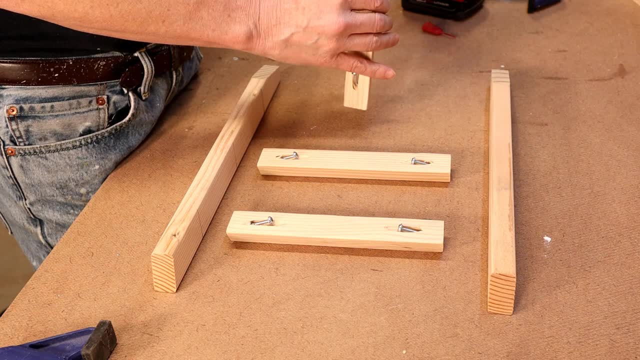 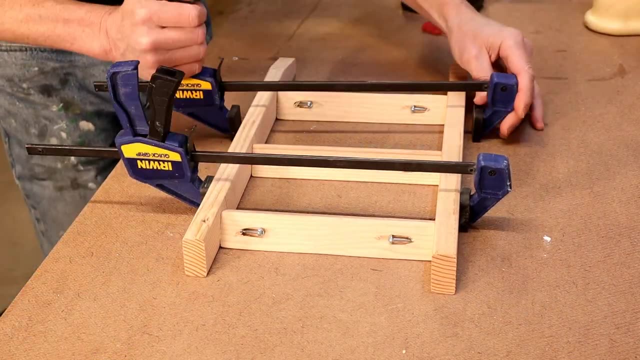 marks and gluing and screwing in the pocket hole screws, I end up with a tea towel ladder, or countertop ladder, as they're sometimes called. I took 80 cents worth of material and in under an hour transformed it into a piece that's worth. 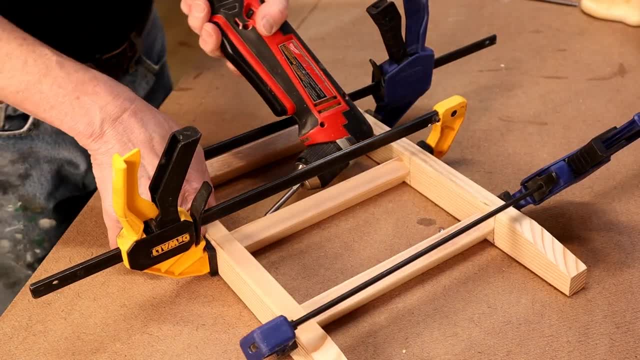 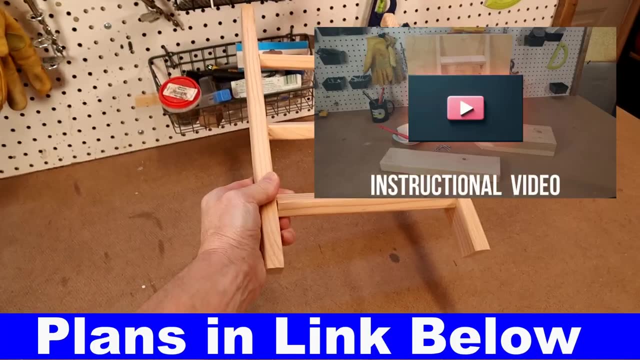 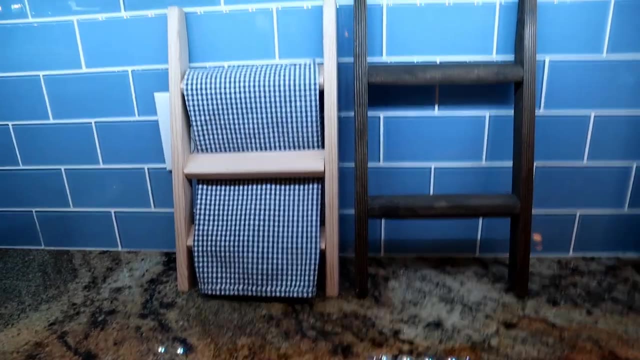 31 times that amount. Now. this would make a great gift, or you could make some extra money by selling them. I put a link below to plans for these ladders. that also includes a private instruction video where I go into much more detail on how to build these and the simple angle cutting jig. So I've seen them on.